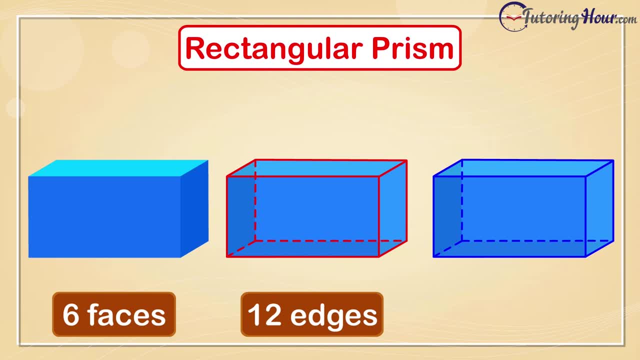 is called a corner or vertex. Let's find out how many vertices there are in a rectangular prism. There are 1,, 2,, 3,, 4,, 5,, 6,, 7, and 8 corners or vertices. 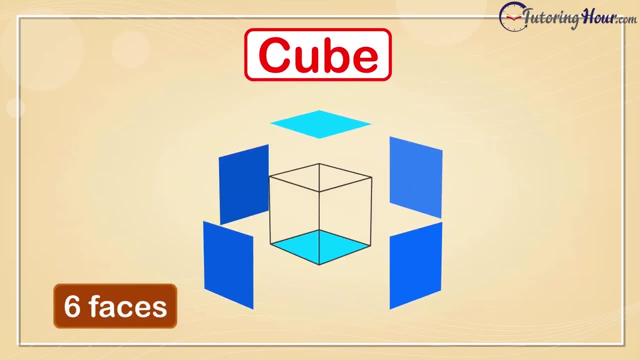 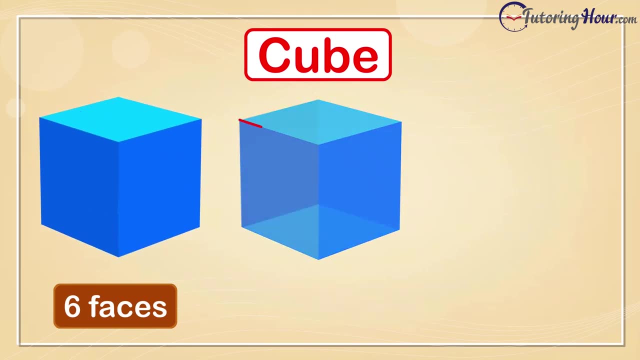 Let's move on to our next prism, the cube. The six identical faces of the cube make it a special rectangular prism. Let's find out how many edges there are in a cube. It has 12 edges. Let's find out the number of vertices it has. 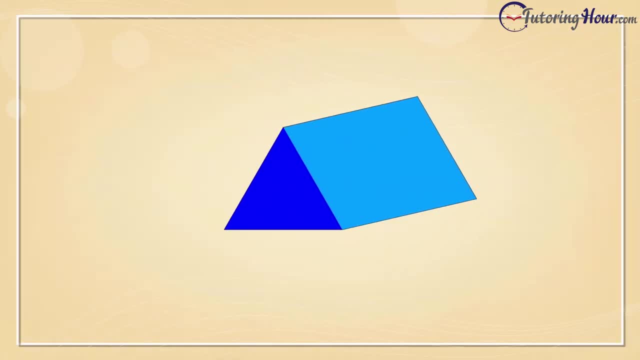 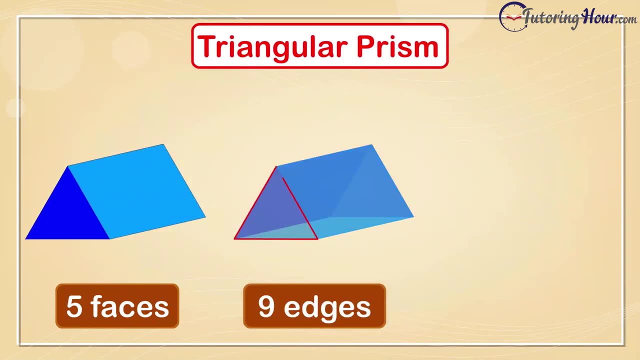 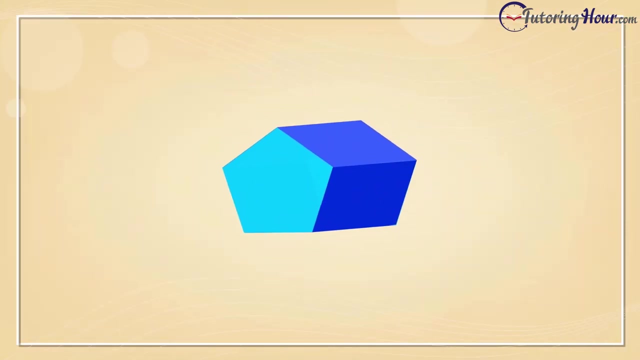 There are 8 vertices here. What's next? A triangular prism. It has 5 faces. A triangular prism has 9 edges. There are 6 vertices or corners. Coming up next is another solid shape: the pentagonal prism. It has 7 faces. 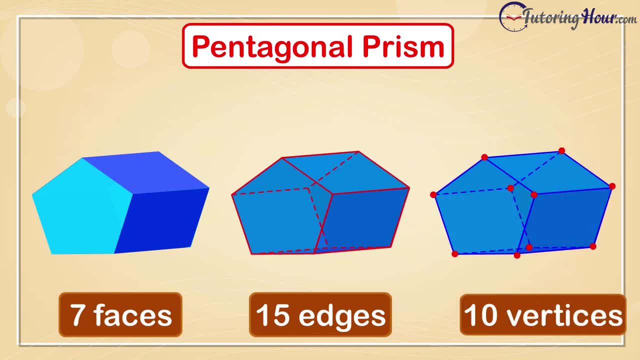 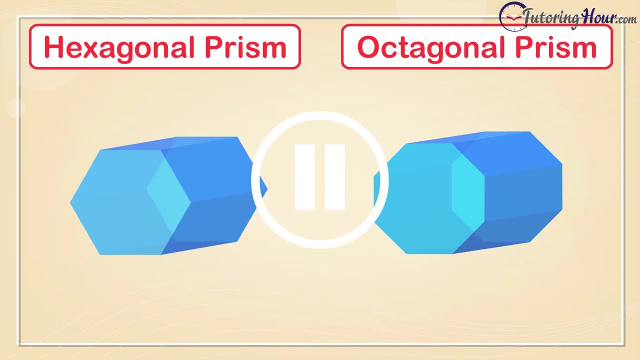 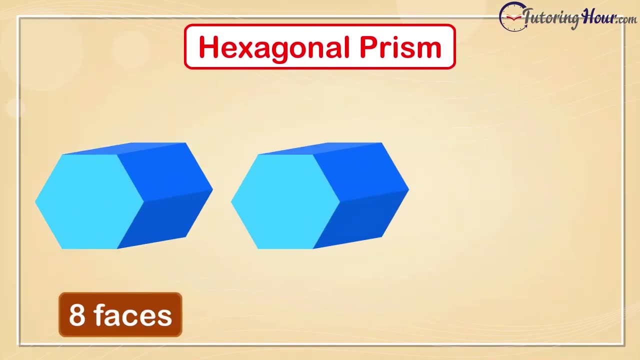 A pentagonal prism players 15 edges. It has 10 vertices. Pause the video. take a look at hexagonal and octagonal prisms and write down the number of faces, edges and vertices in them. A hexagonal prism has 8 faces, 18 edges and 12 vertices. 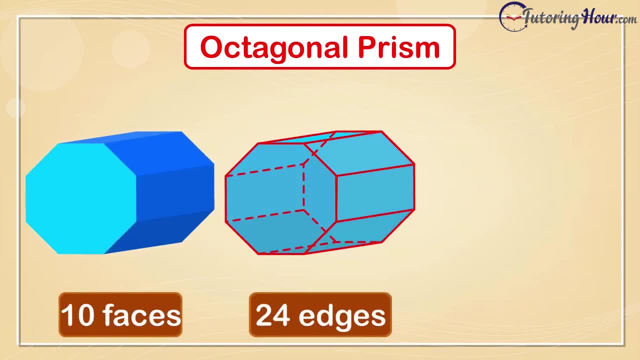 An octagonal prism has 10 faces, 24 edges and 16 vertices. Final horn: shape number. Give yourself a paddle note like a feather. Let's get startedziest page: Folk, meine erste erhaut walking Note the number of faces, edges and vertices. An octagonal picture has 9 faces and 16 edges and vertices. Tell them all that you have the number of faces. 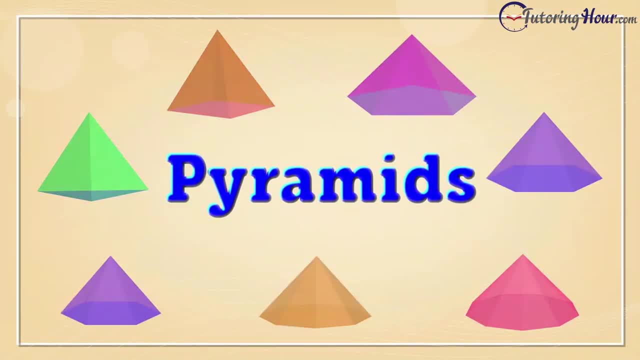 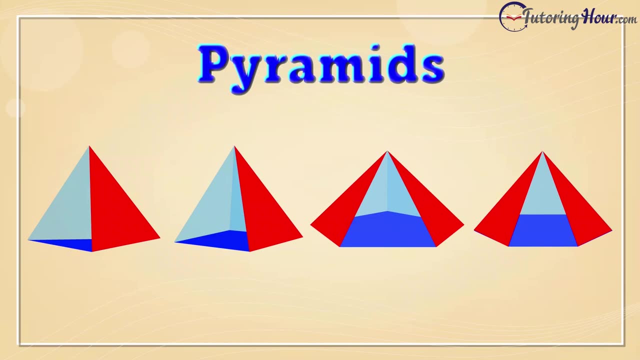 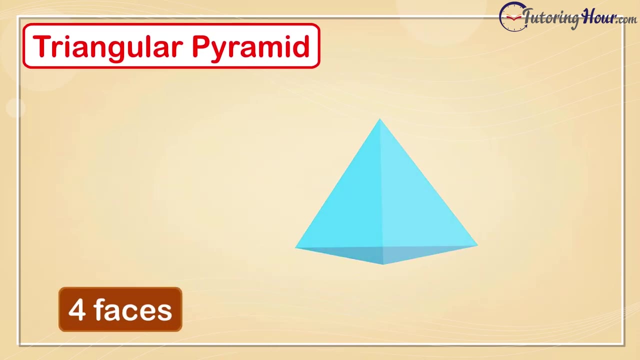 the back for getting them right. let's move on to the pyramids. all pyramids have a base and vertex. all its side faces are triangles. pyramids are named after the shape of their bases. let's take a look at our first pyramid, the triangular pyramid. it has four faces. it has 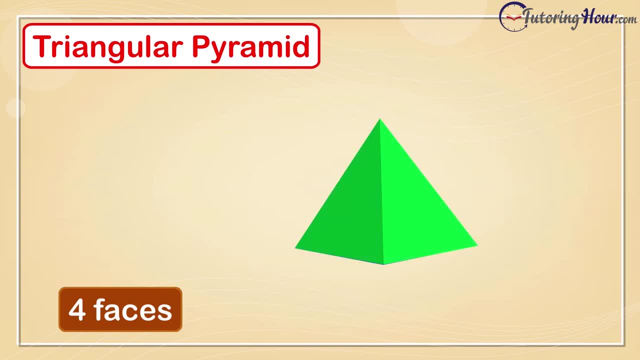 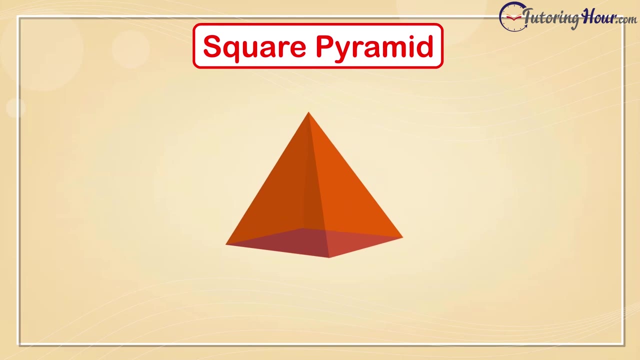 one triangular base in three triangular side faces. a triangular pyramid has six edges. it is four vertices. our next pyramid has a square base. no points for guessing its name: it is a square pyramid. a square pyramid has five faces. it has a square base and four triangular side faces. 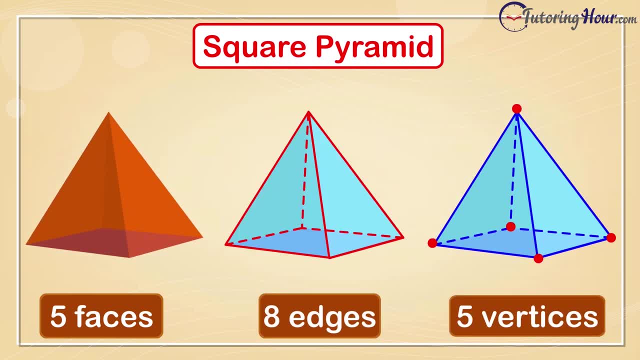 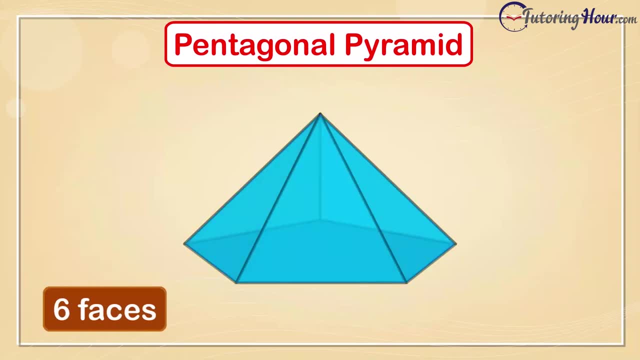 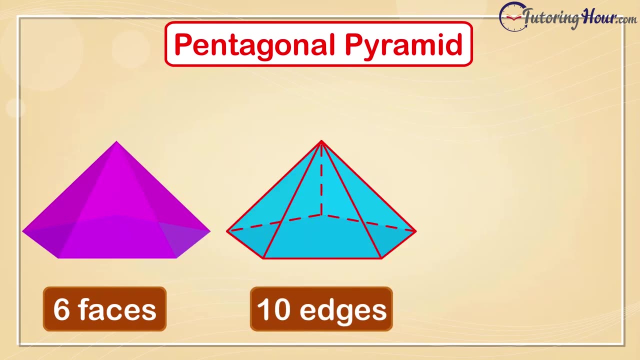 a square pyramid has eight edges. it has five vertices. up next is the pentagonal pyramid. a pentagonal pyramid has six spaces. it has a pentagonal base and five triangular side faces. a pentagonal pyramid has ten edges. it has six vertices. let's take a look at the. 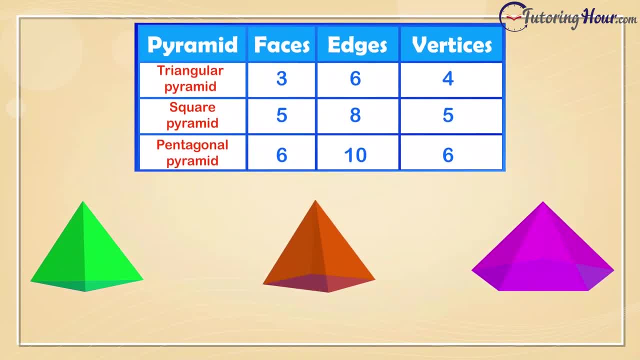 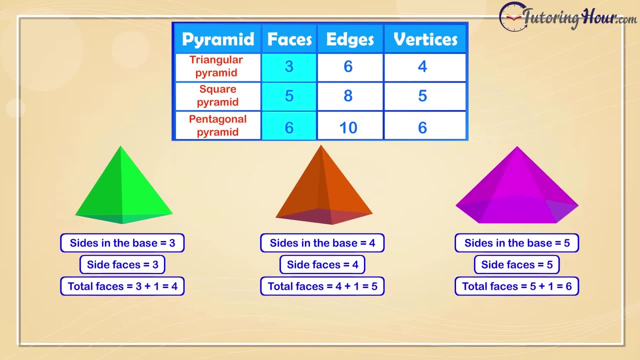 faces, edges and vertices of the three pyramids. do you see a pattern? the number of side faces is the same as the number of sides in the base. the total number of faces is the number of sides in the base plus one. the number of edges is twice the number of sides in the base. 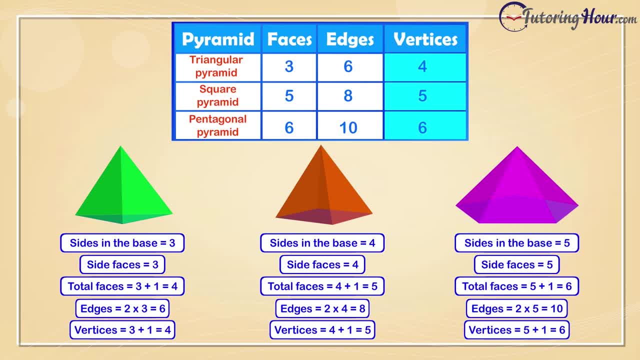 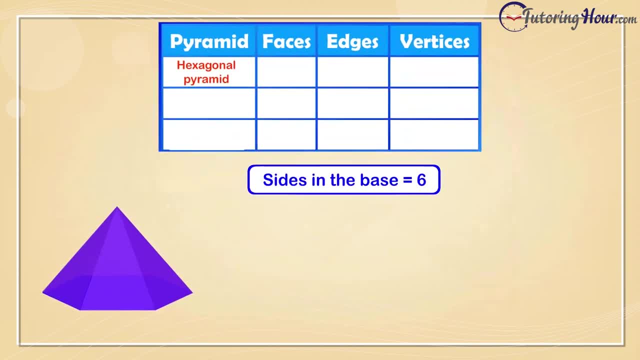 the number of vertices is the number of sides in the base plus one. let's use this little trick and quickly fill up the faces, edges and vertices of the hexagonal pyramid. The base of a hexagonal pyramid is obviously a hexagon. It has 6 sides and the number of faces is 6 plus 1, so we have 7 here. 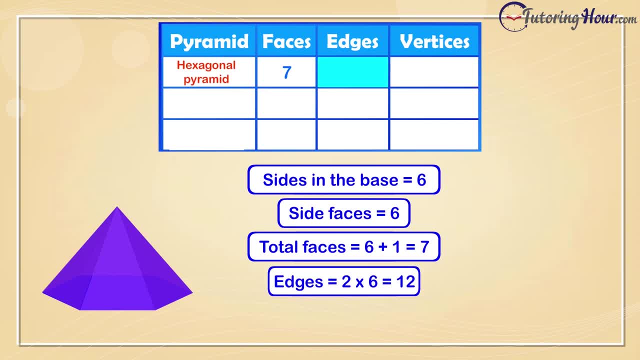 The number of edges is twice the number of sides and the base, so we'll write 12 here. The number of vertices is the number of sides and the base plus 1, so we'll write 7 here as well. We'll quickly do the same for the heptagonal and octagonal pyramids. 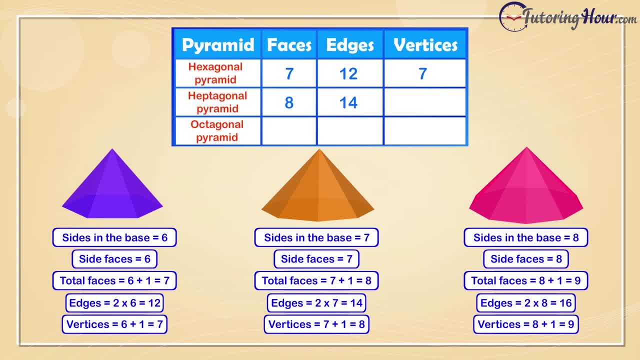 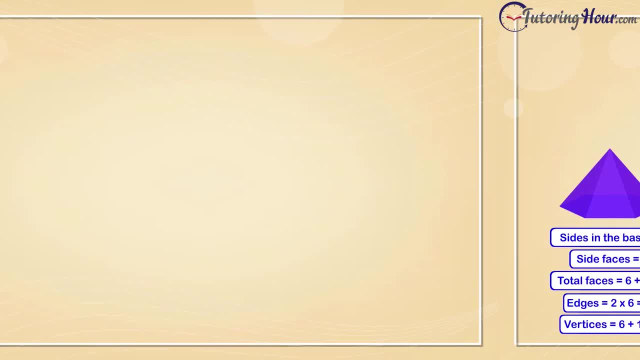 A heptagonal pyramid has 8 faces, 14 edges and 8 vertices, and an octagonal pyramid has 9 faces, 16 edges and 9 vertices. Let's move on to solid shapes with curved surfaces. Here comes the cylinder, our next solid shape. 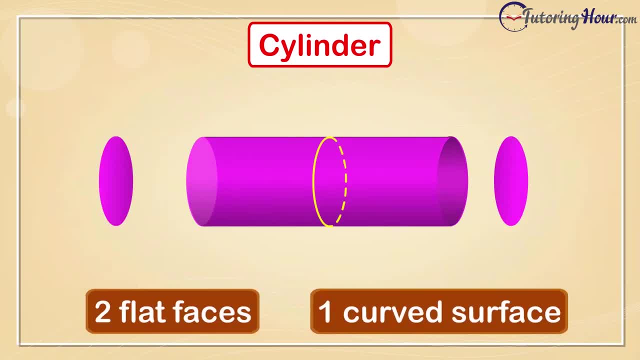 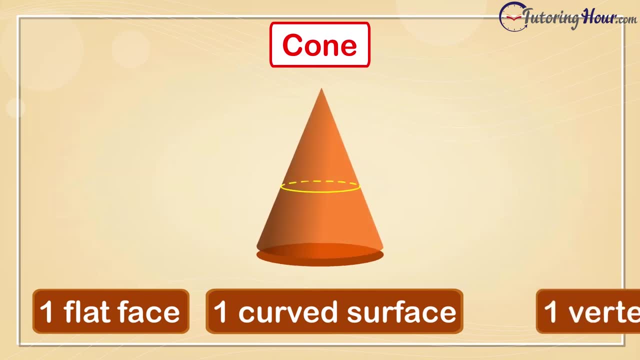 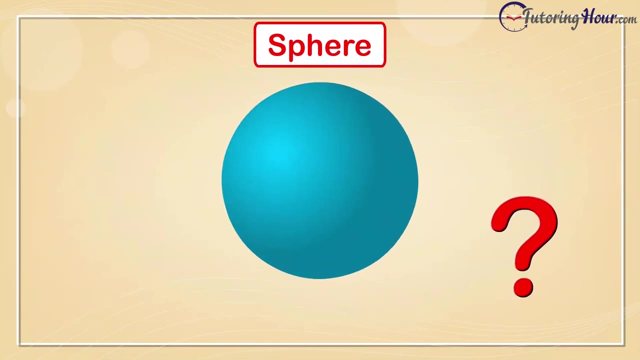 A cylinder has two flat faces and a curved surface. Let's meet our next shape, the cone. A cone has one flat face and one curved surface. It has one vertex. Here comes our last shape, the sphere. How many edges and vertices do you see here? 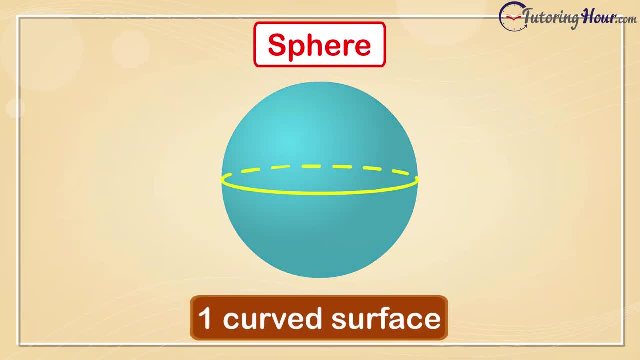 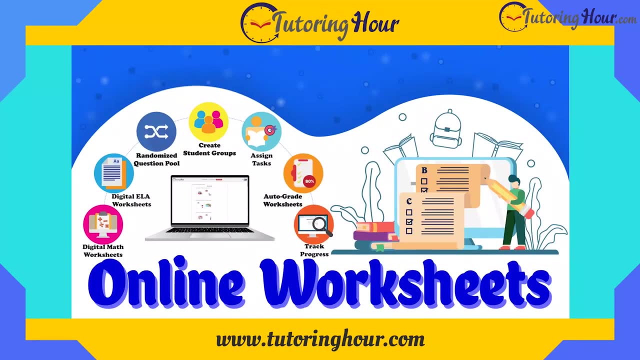 A sphere has no edges or vertices. It has just one curved surface. That was quite a lot of information. If you want to put your newfound knowledge to the test, visit wwwtutoringhourcom for practice worksheets, Smash the like and subscribe buttons and show us some love. Thanks for watching, Bye-bye.